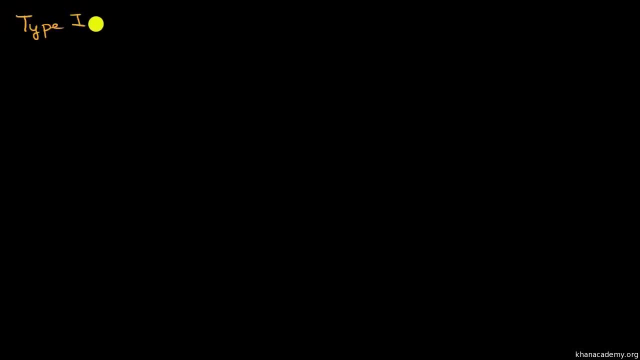 What we're going to do in this video is talk about type one errors and type two- type two errors, And this is in the context of significance testing. So, just as a little bit of review: in order to do a significance test, we first come up with a null and an alternative hypothesis. 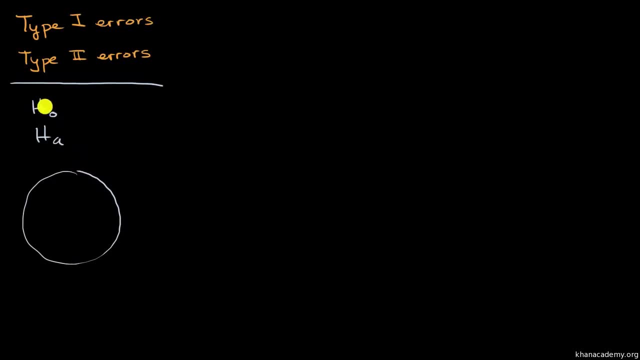 And we'll do this on some population in question. These will say some hypotheses about a true parameter for this population, And the null hypothesis tends to be kind of what was always assumed or the status quo, while the alternative hypothesis- hey, there's news here. 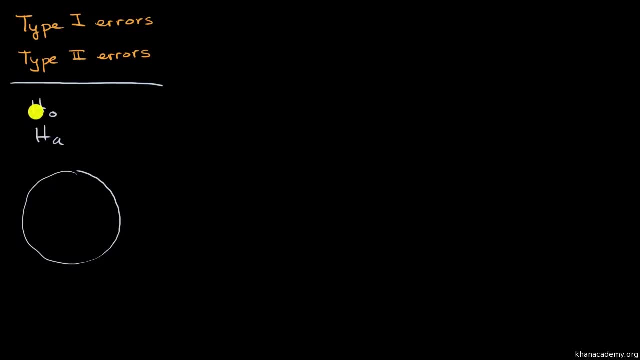 There's something alternative here, And to test it- and we're really testing the null hypothesis- We're gonna decide whether we want to reject or fail to reject the null hypothesis. We take a sample. We take a sample from this population. Using that sample, we calculate a statistic. 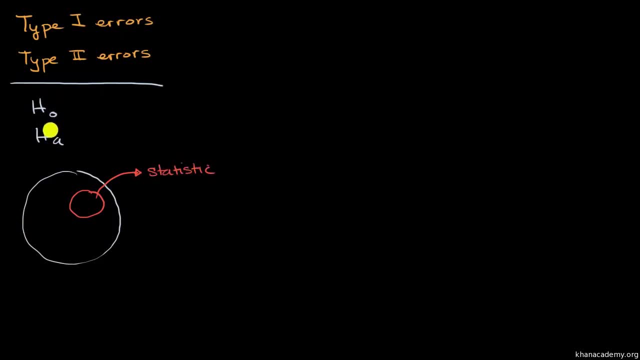 We calculate a statistic that's trying to estimate the parameter in question And then, using that statistic, we try to come up with the probability of getting that statistic, the probability of getting that statistic that we just calculated from that sample of a certain size. 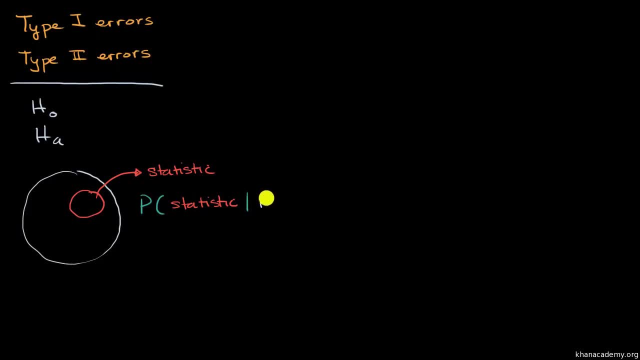 given if we were to assume that our null hypothesis, if our null hypothesis is true And if this probability, which is often known as a p-value, is below some threshold that we set ahead of time, which is known as the significance level? 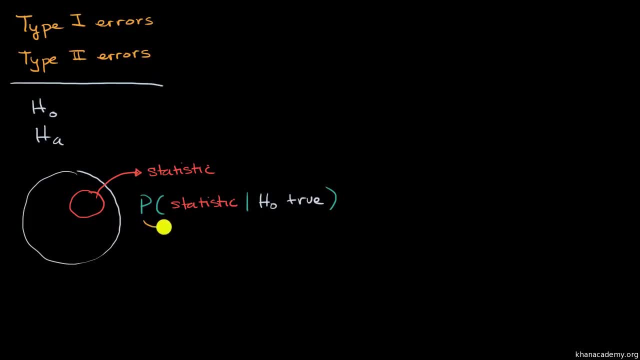 then we reject the null hypothesis. Let me write this down. So this right over here: this is our p-value. This should all be review. We introduce it in other videos. We have seen in other videos: if our p-value is less than our significance level, 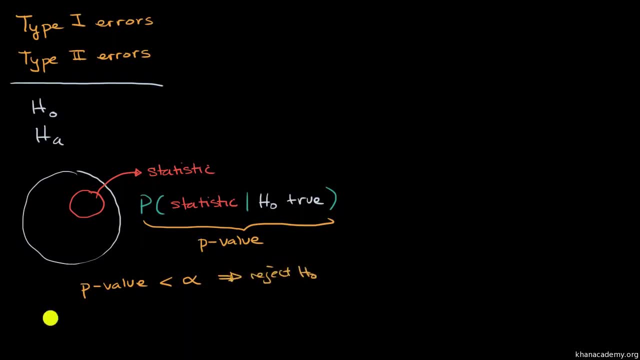 then we reject our null hypothesis. And if our p-value is greater than or equal to our significance level alpha, then we fail to reject, fail to reject our null hypothesis. And when we reject our null hypothesis, some people will say that might suggest. 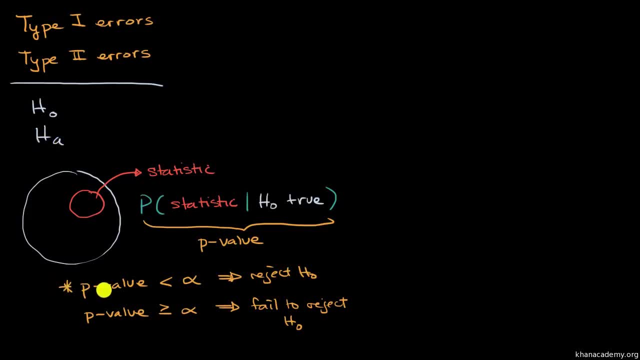 the alternative hypothesis, And the reason why this makes sense is if the probability of getting this statistic from a sample of a certain size- if we assume that the null hypothesis is true- is reasonably low. if it's below a threshold, maybe this threshold is five five, five, five, five, five. 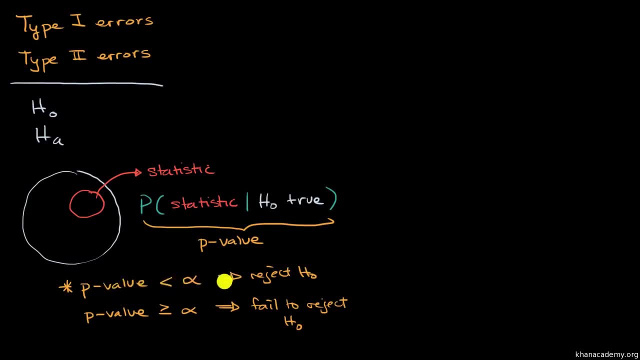 five percent. if the probability of that happening was less than five percent, then hey, maybe it's reasonable to reject it, But we might be wrong in either of these scenarios, and that's where these errors come into play. Let's make a grid to make this clear. 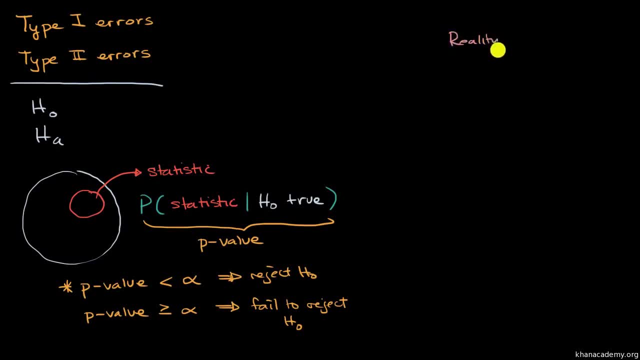 So there's the reality. Let me put reality up here. So the reality is there's two possible scenarios in reality. One is: is that the null hypothesis is true, and the other is that the null hypothesis is false and then based on our significance test. 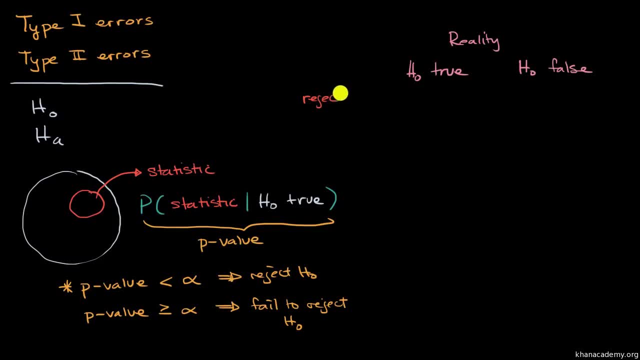 there's two things that we might do. We might reject the null hypothesis or we might fail to reject the null hypothesis, And so let's put a little grid here to think about the different combinations, the different scenarios here. So, in a scenario where the null hypothesis is true, 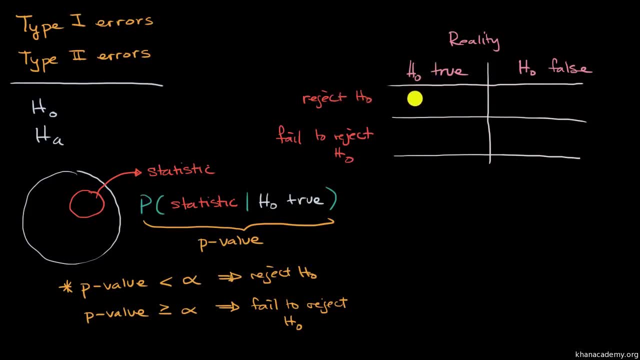 but we reject it. that feels like an error. We shouldn't reject something that is true And that, indeed, is a type I error. Type I error. You shouldn't reject the null hypothesis if it was true And you can even figure out what is the probability. 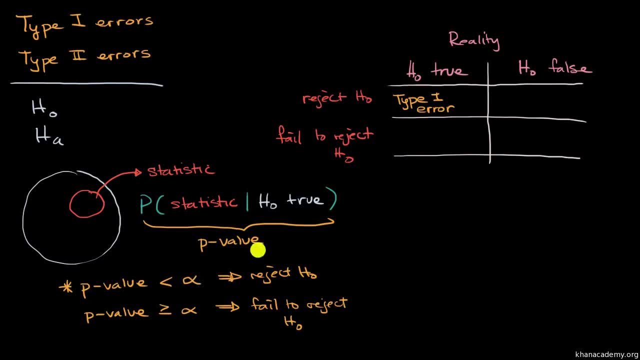 of getting a type I error. Well, that's gonna be your significance level, Because if your null hypothesis is true, let's say that your significance level is five percent. Well, five percent is庸. even if your null hypothesis is true, you're going to get a statistic. 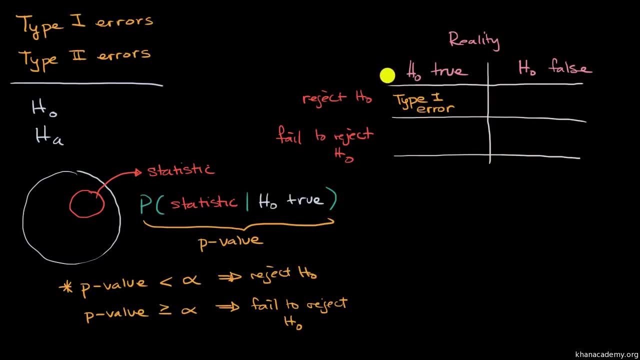 that's going to make you reject the null hypothesis. So one way to think about the probability of a type one error is your significance level. Now, if your null hypothesis is true and you fail to reject it, well, that's good This. we could write this as: